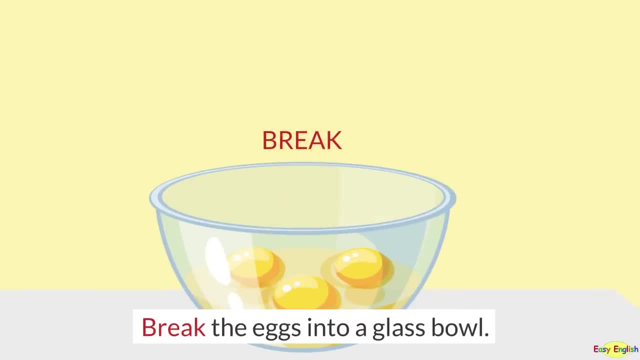 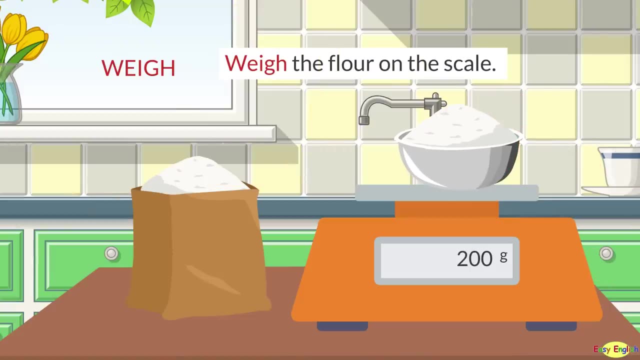 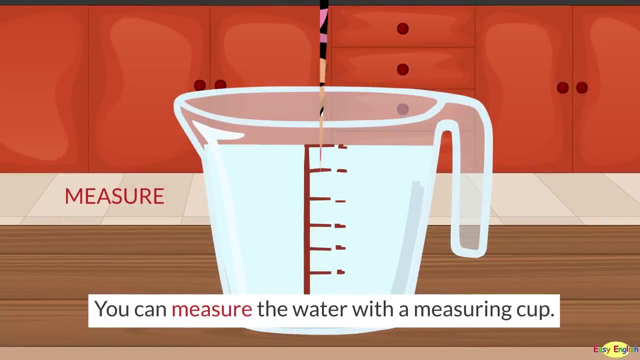 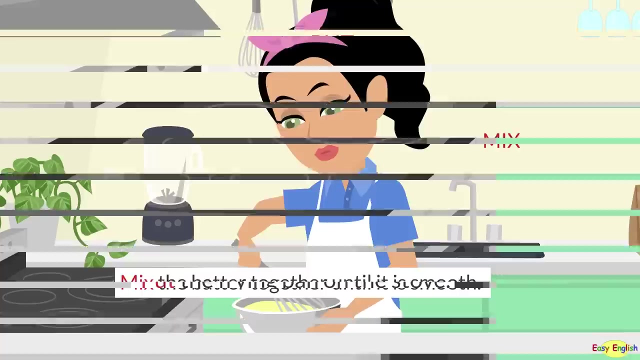 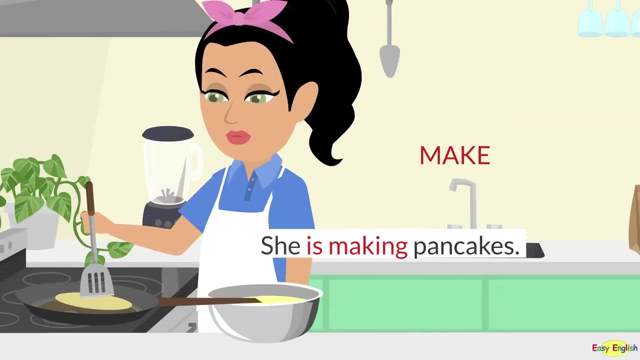 Break. Break the eggs into a glass bowl. Weigh. Weigh the flour on the scale. Measure- You can measure the water with a measuring cup. Mix, Mix the batter together until it is smooth. Put, Put the frying pan on the stove. Make- She is making pancakes. 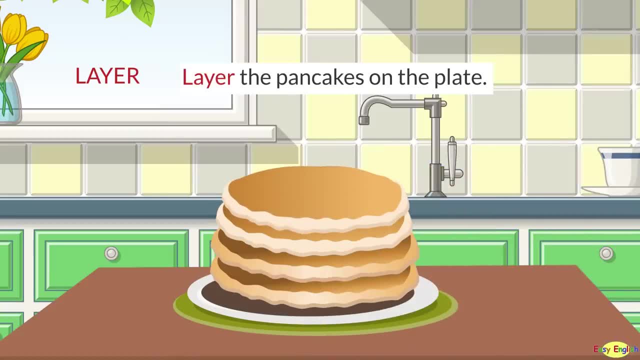 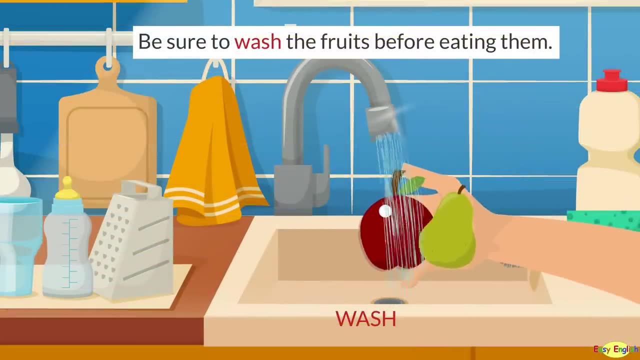 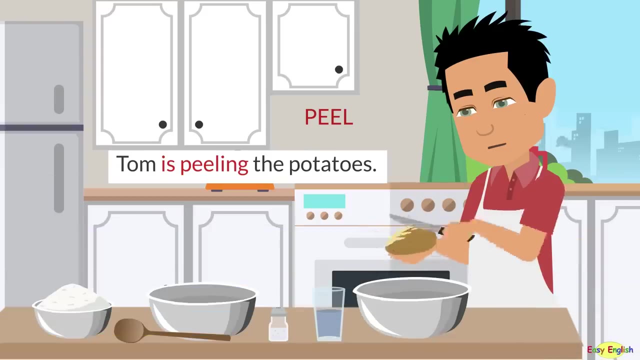 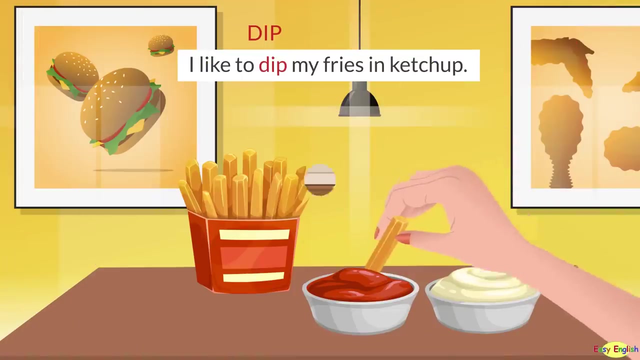 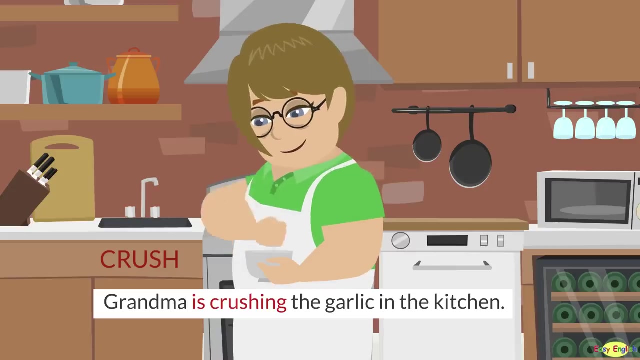 Layer. Layer the pancakes on the plate. Wash- Be sure to wash the fruits before eating. Peel Tom is peeling the potatoes. Dice, Dice the potatoes into cubes Dip: I like to dip my fries in ketchup Crush. Grandma is crushing the garlic in the kitchen. 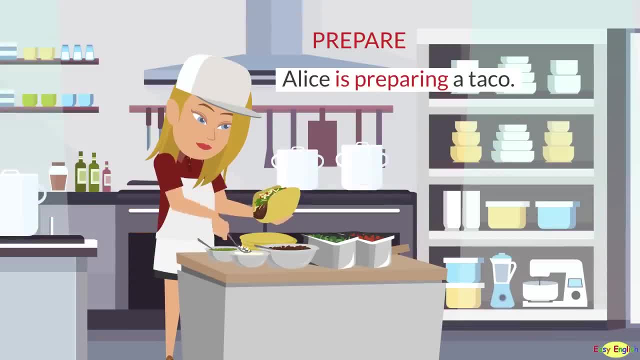 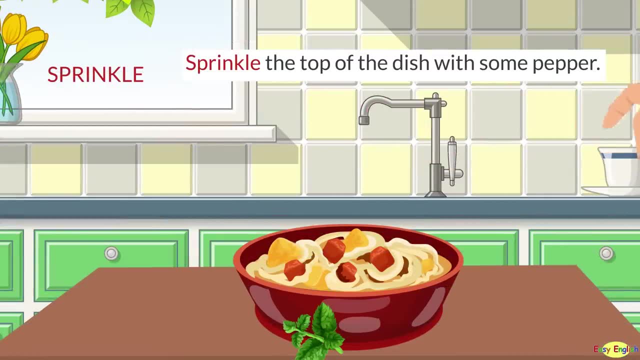 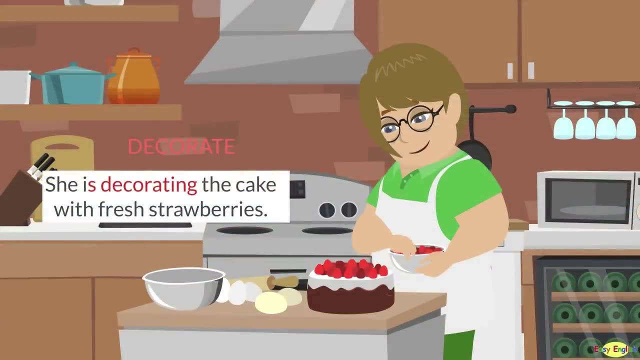 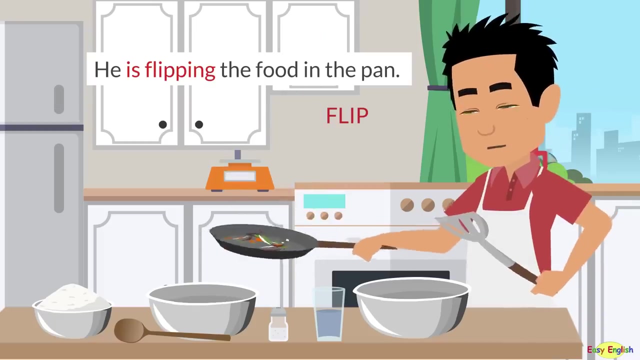 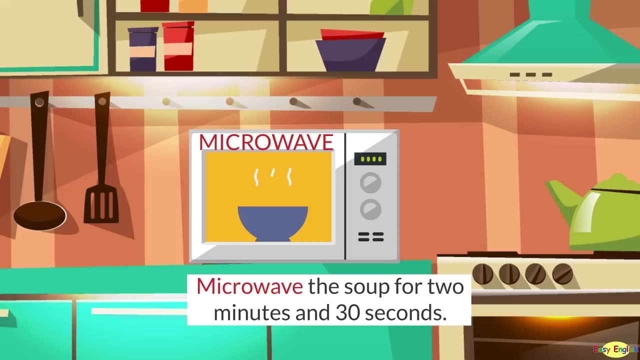 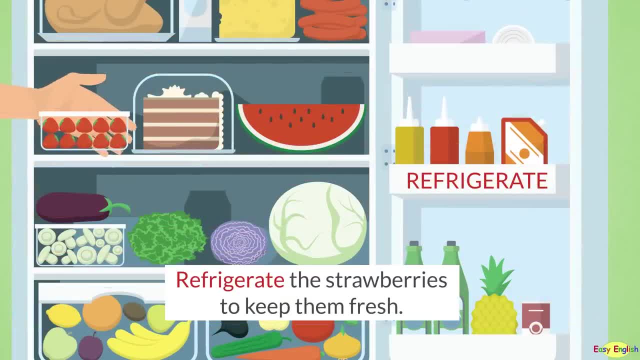 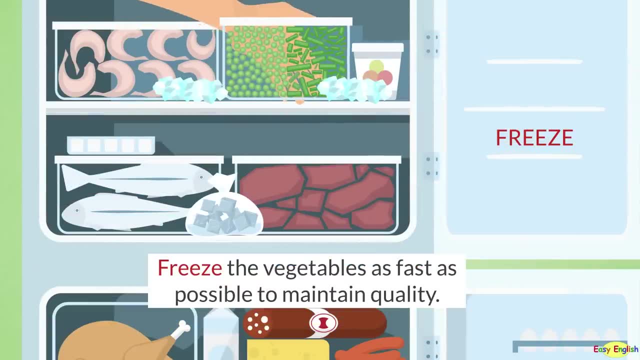 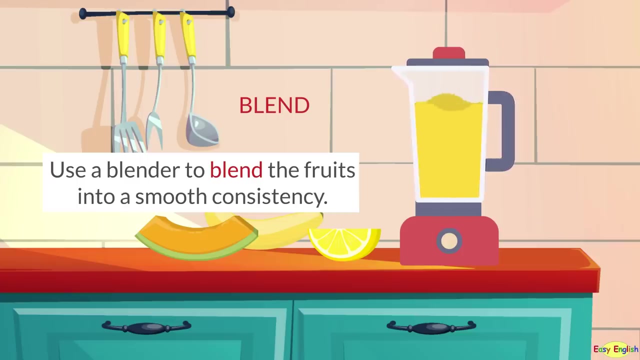 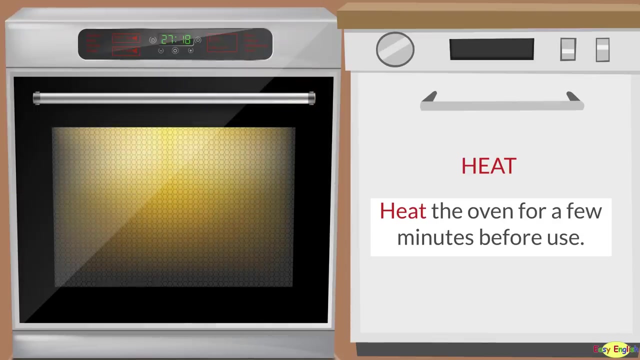 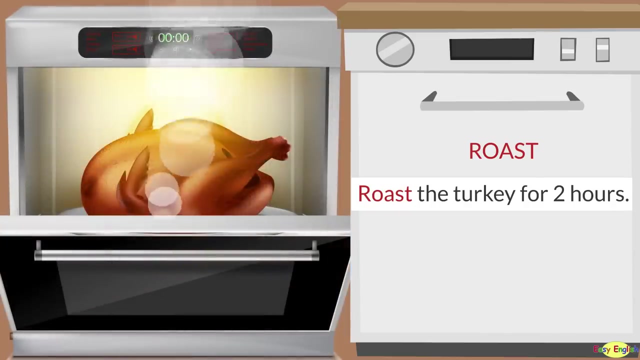 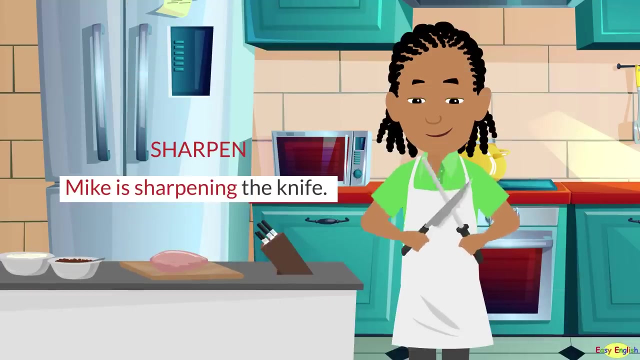 refrigerate. refrigerate the strawberries to keep them fresh. freeze. freeze the vegetables as fast as possible to maintain quality. blend: use a blender to blend the fruits into a smooth consistency. heat: heat the oven for a few minutes before you use Roast. Roast the turkey for two hours. Sharpen- Mike is sharpening the knife. Add: 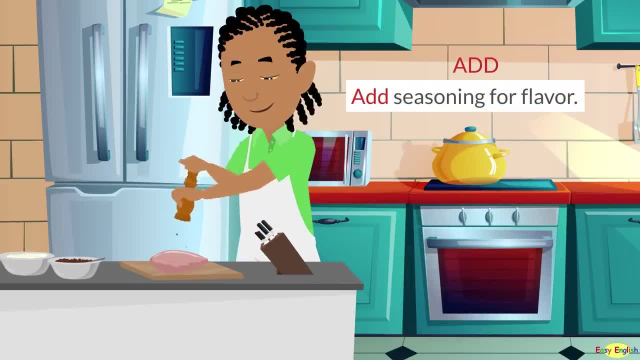 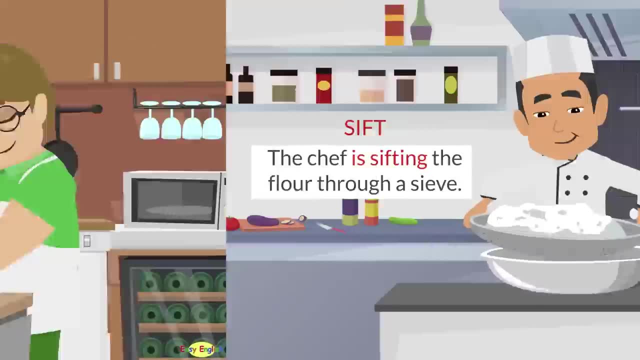 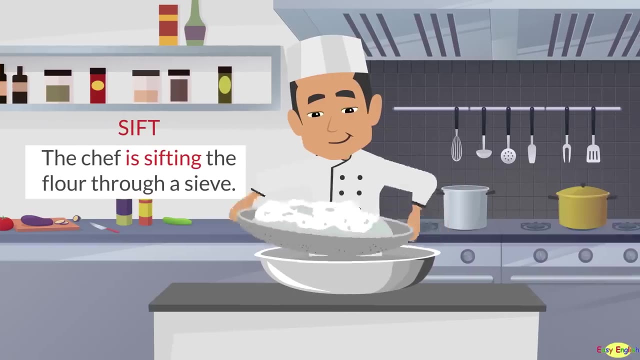 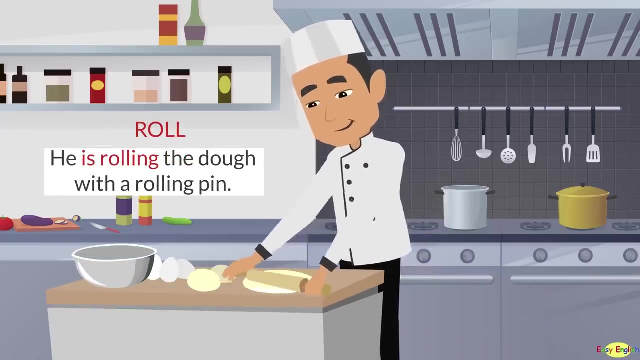 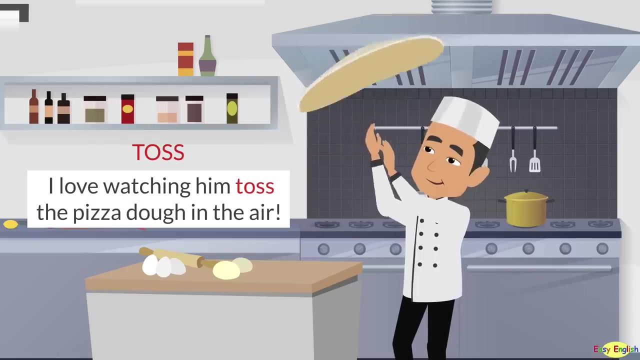 Add seasoning for flavor. Cut: She is cutting the fish into small pieces. Sift: The chef is sifting the flour through a sieve. Roll: He is rolling the dough with a rolling pin. Toss: I love watching him toss the pizza dough in the air. Great, I am grating. 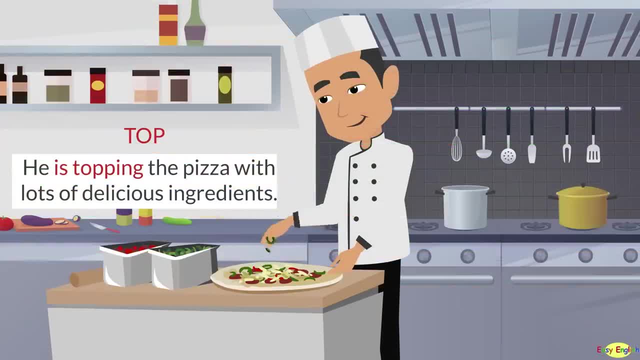 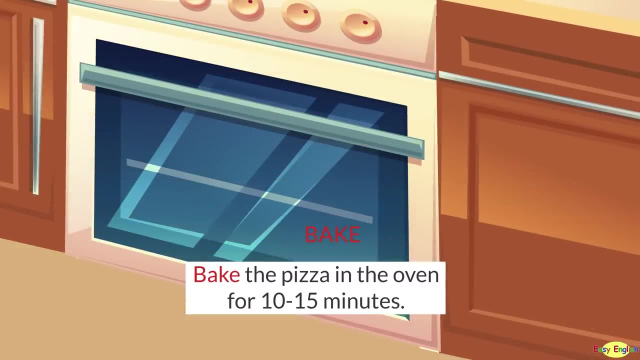 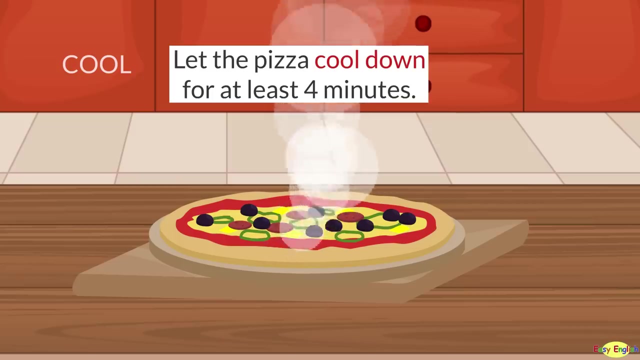 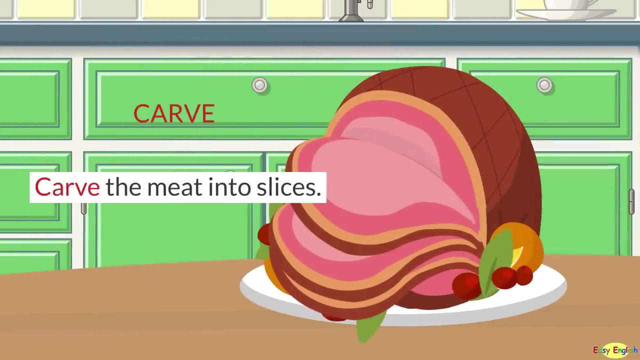 the cheese for the pizza Top. He is topping the pizza. Top the pizza with lots of delicious ingredients. Bake. Bake the pizza in the oven for ten to fifteen minutes. Cool. Let the pizza cool down for at least four minutes. Carve. Carve the meat into slices. Mash. Mash the potatoes with a fork. 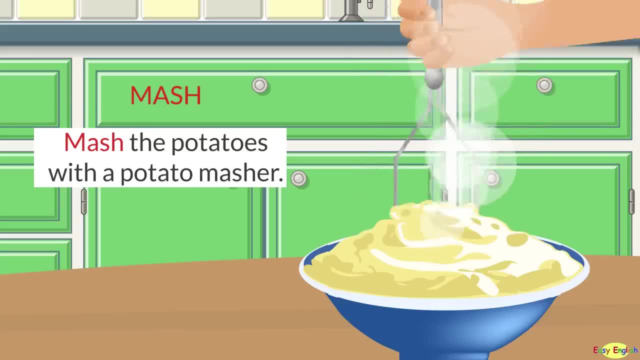 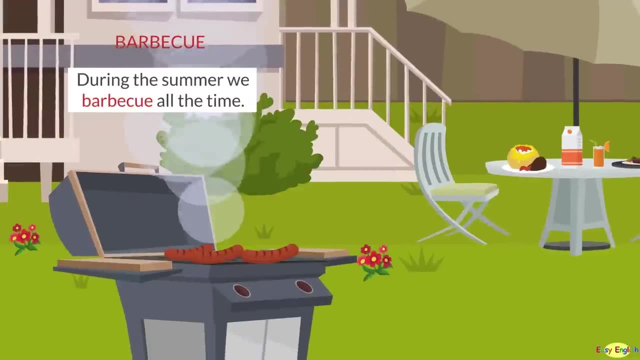 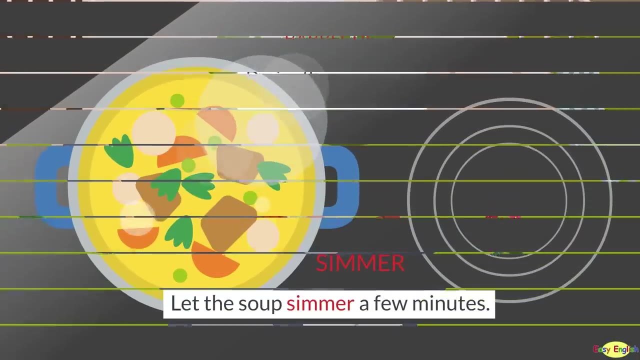 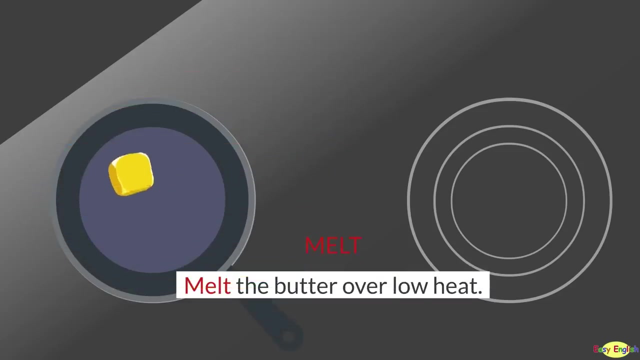 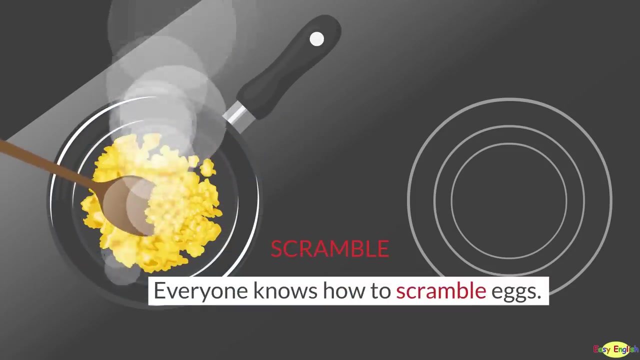 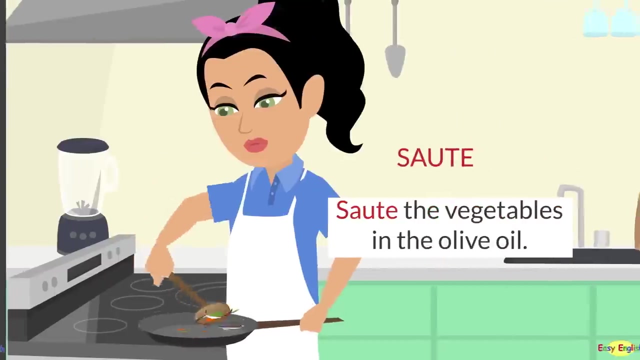 Tenderize. Tenderize the meat with a meat tenderizer. Barbecue- During the summer we barbecue all the time. Simmer- Let the soup simmer a few minutes. Melt: Melt the butter over low heat. Fry- I am frying an egg Scramble. Everyone knows how to scramble eggs. Saute. Saute the. 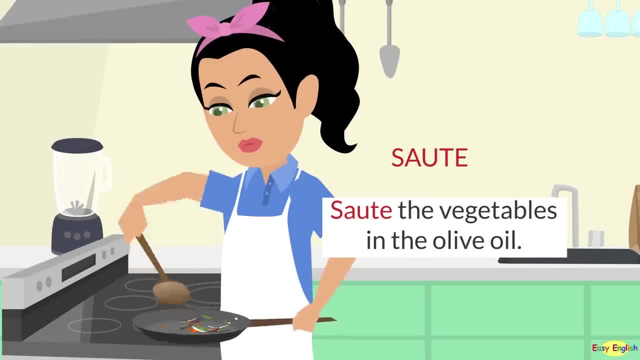 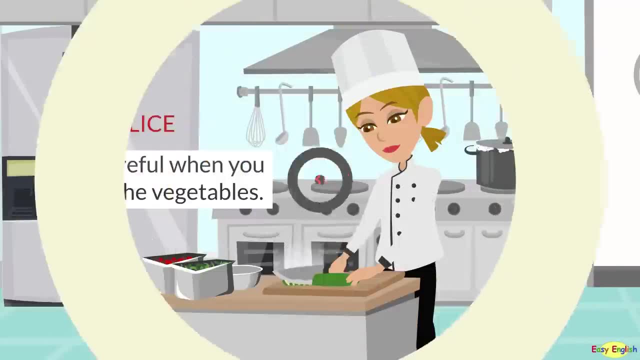 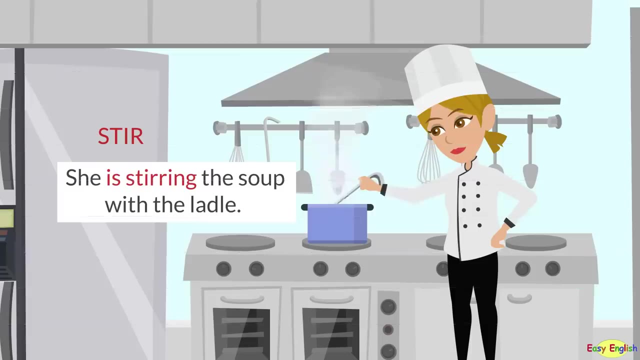